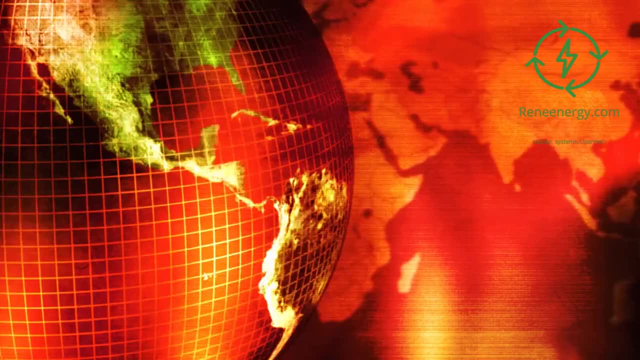 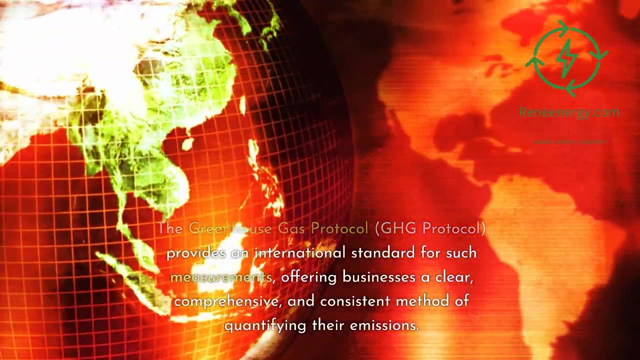 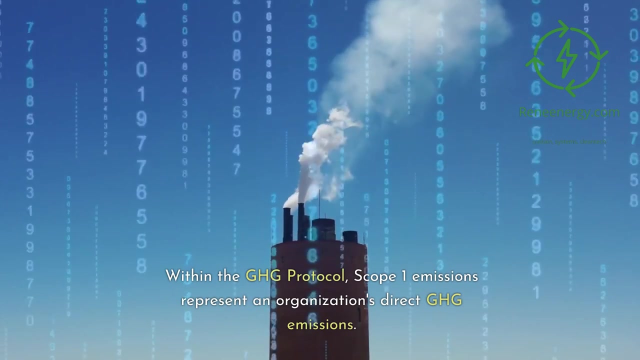 greenhouse gas emissions. The Greenhouse Gas Protocol provides an international standard for such measurements, offering businesses a clear, comprehensive and consistent method of quantifying their emissions. Within the GHG protocol, Scope 1 emissions represent an organization's direct GHG emissions. These emissions come from sources owned or controlled. 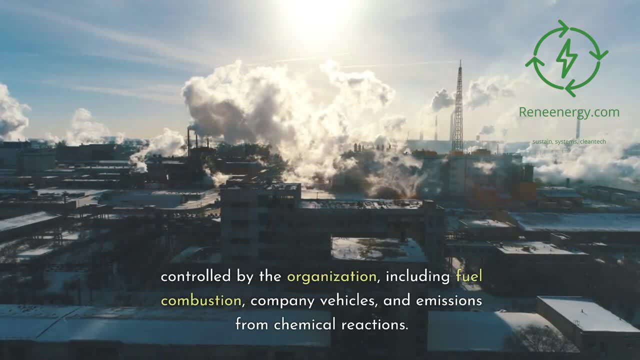 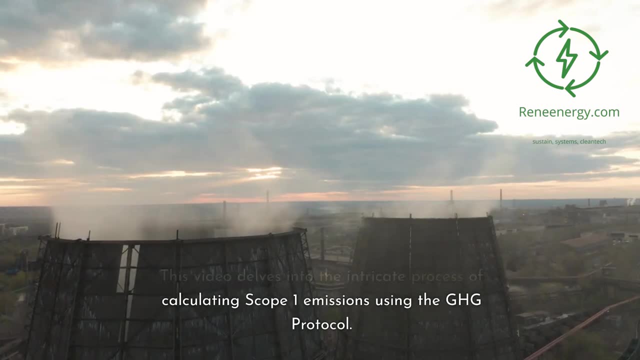 by the organization. In the GHG protocol, Scope 1 emissions represent an organization's direct GHG emissions. These emissions come from sources owned or controlled by the organization, including fuel combustion company vehicles and emissions from chemical reactions. This video delves into the intricate process of calculating Scope 1 emissions using the GHG. 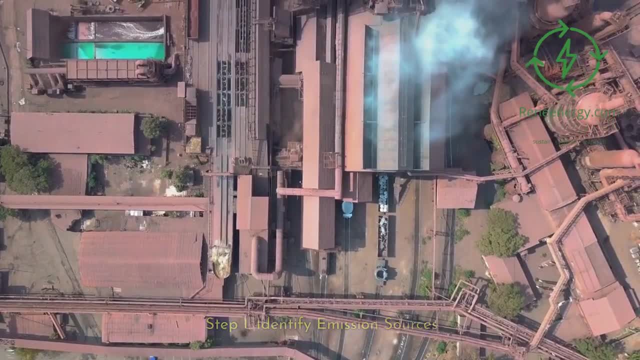 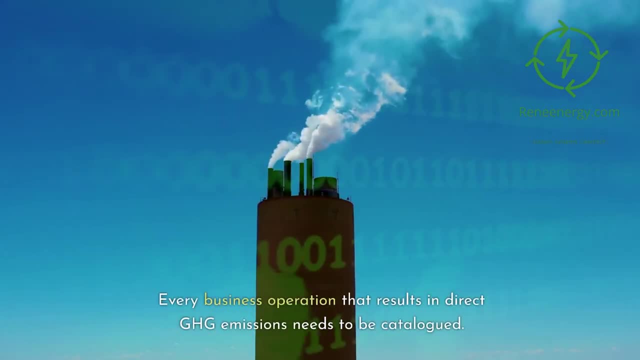 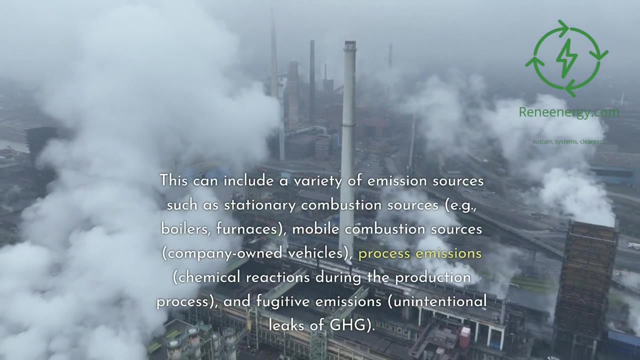 protocol, Step 1. Identify Emission Sources. The first step in Scope 1 emissions calculations is the identification of emission sources. Every business operation that results in direct GHG emissions needs to be catalogued. This can include a variety of emission sources, such as stationary combustion sources, for example. boilers, gas stoves, gas stoves, etc. This can include a variety of emission sources, such as stationary combustion sources, for example, boilers, gas stoves, gas stoves, etc. Boilers, furnaces- mobile combustion sources. 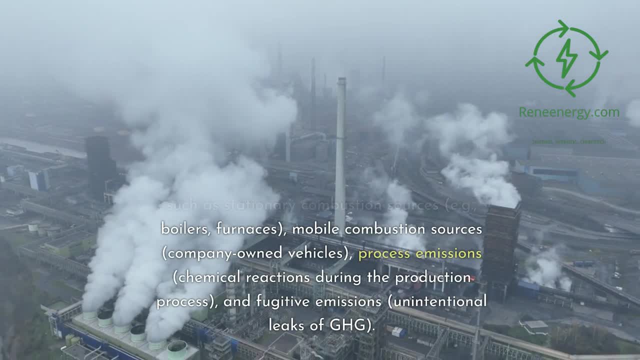 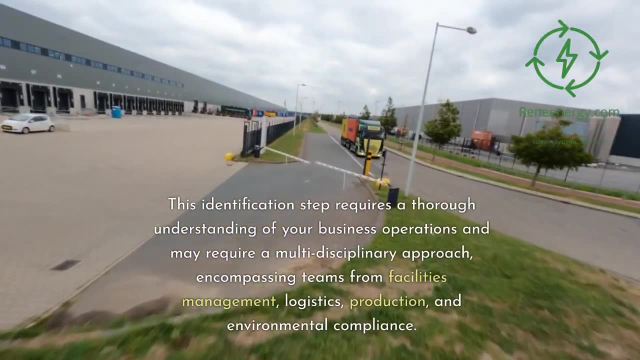 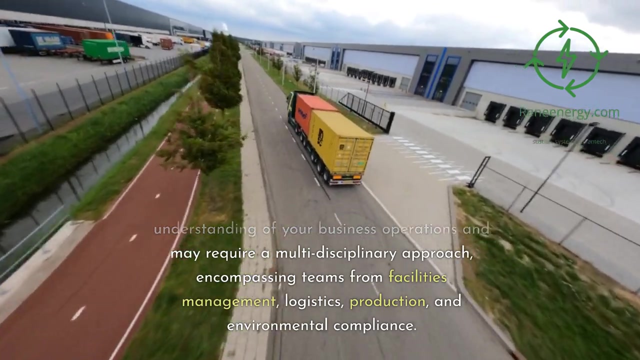 company-owned vehicles. process emissions, chemical reactions during the production process and fugitive emissions. unintentional leaks of GHG. This identification step requires a thorough understanding of your business operations and may require a multidisciplinary approach encompassing teams from facilities management. 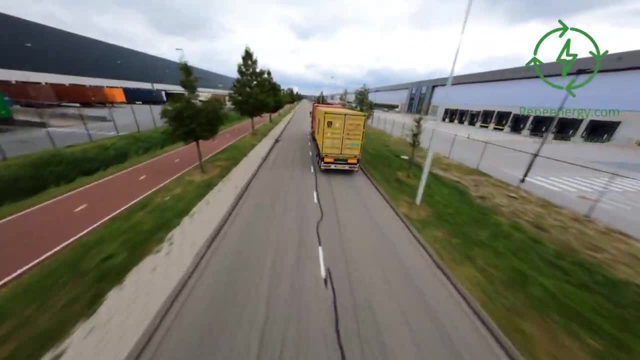 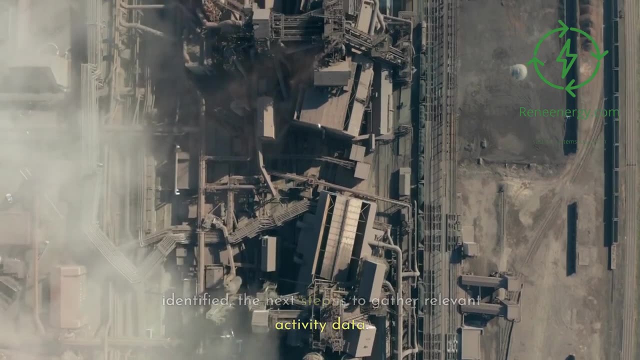 logistics, production and environmental compliance. Step 2. Gather Activity Data. Once the emission sources have been identified, the next step is to collect data. The next step is to gather relevant activity data. This data pertains to the quantity of activities. 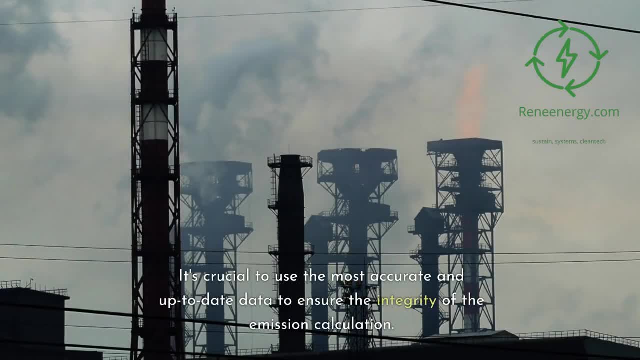 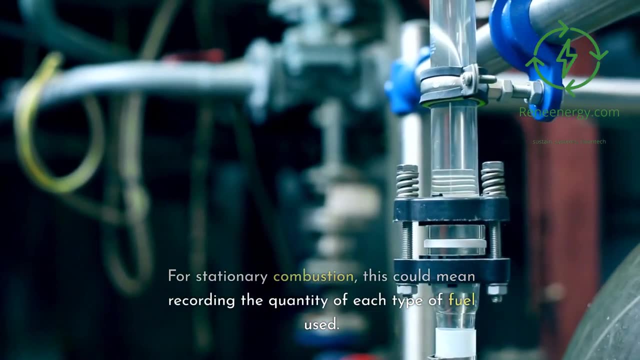 resulting in emissions. It's crucial to use the most accurate and up-to-date data to ensure the integrity of the emission calculation. For stationary combustion, this could mean recording the quantity of each type of fuel used. Mobile combustion would necessitate data such as the: 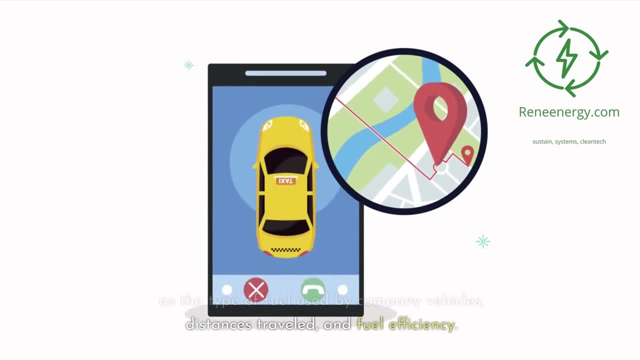 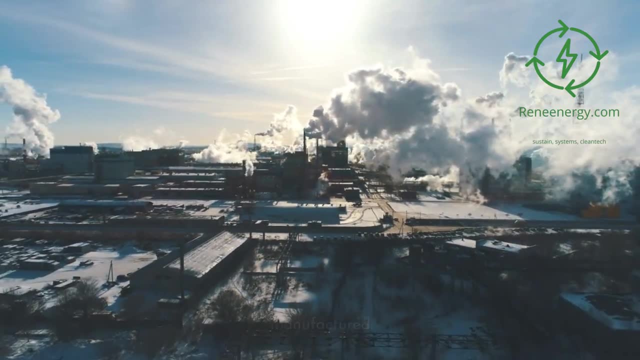 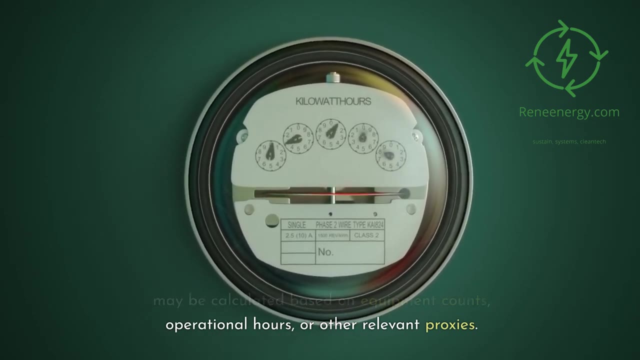 type of fuel used by company vehicles, distances traveled and fuel efficiency. Process emissions calculations require the quantity of raw materials used or products manufactured. Fugitive emissions being harder to measure may be calculated based on equipment counts, operational hours or other relevant proxies. 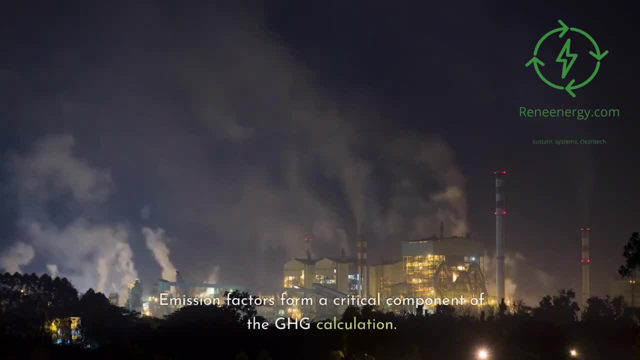 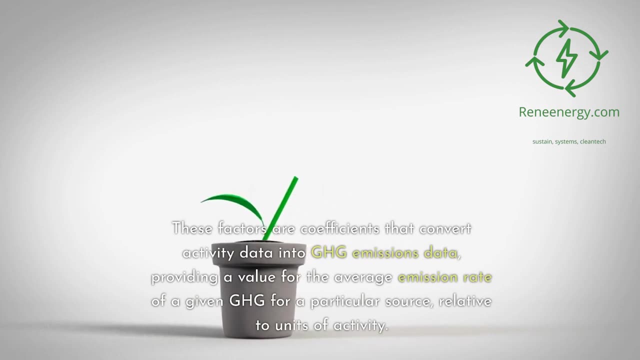 Step 3. Determine Emission Factors. Emission factors form a critical component of the GHG calculation. These factors are coefficients that convert activity data into GHG emissions data, providing a value for the average emission rate of a given GHG for a. 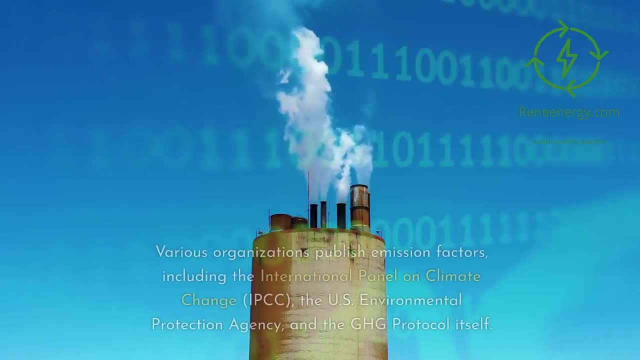 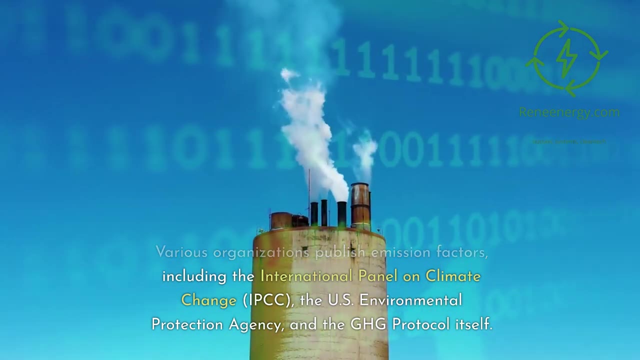 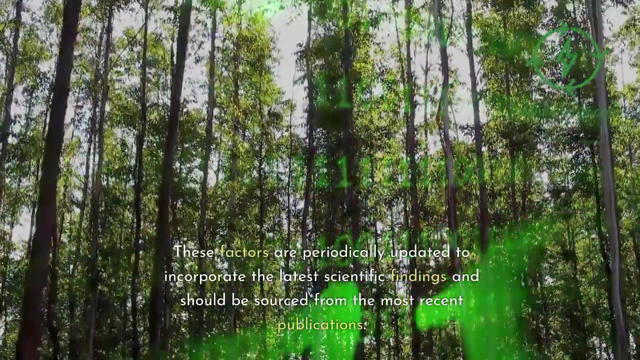 particular source. relative to units of activity, Various organizations publish emission factors, including the International Panel on Climate Change, the US Environmental Protection Agency and the GHG Protocol itself. These factors are periodically updated to incorporate the latest scientific findings and should be sourced from the most recent publications. 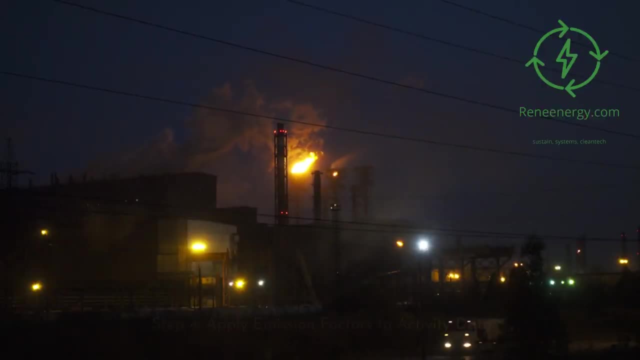 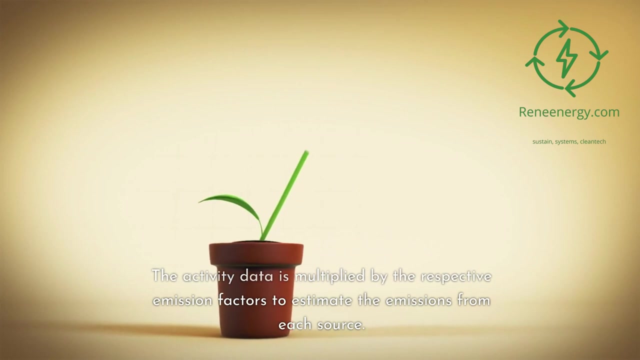 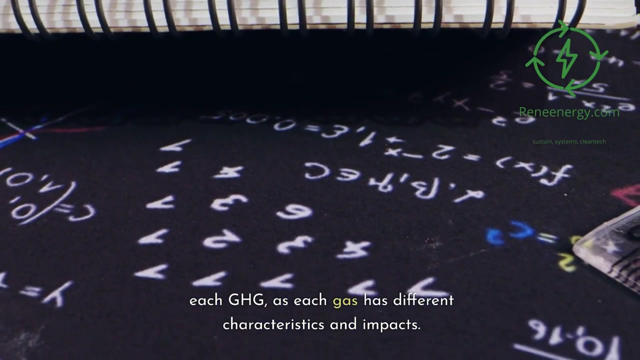 Step 4. Apply Emission Factors to Activity Data. The actual calculation of emissions occurs in this step. The activity data is multiplied by the respective emission factors to estimate the emissions from each source. Calculations should be done separately for each GHG, as each gas has different characteristics and impacts. The 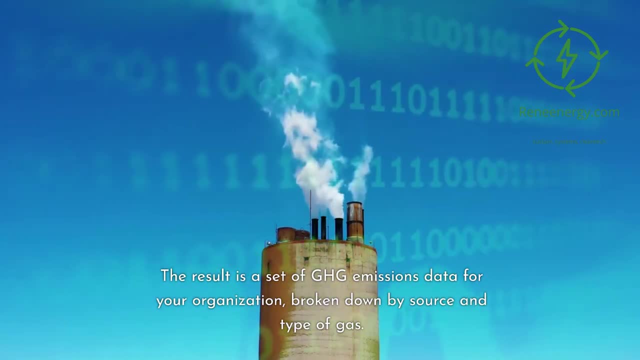 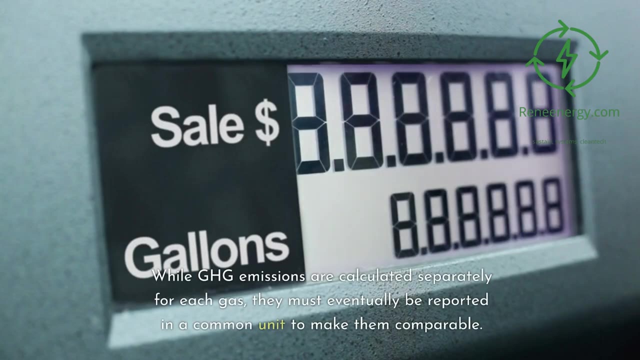 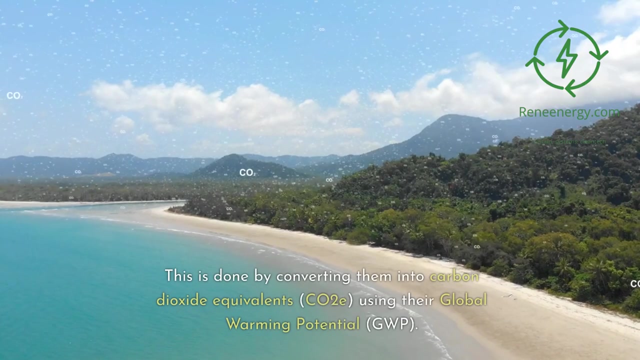 result is a set of GHG emissions data for your organization, broken down by source and type of gas. Step 5. Convert to CO2 Equivalents. While GHG emissions are calculated separately for each gas, they must eventually be reported in a common unit to make them comparable. This is done by converting them into carbon dioxide. 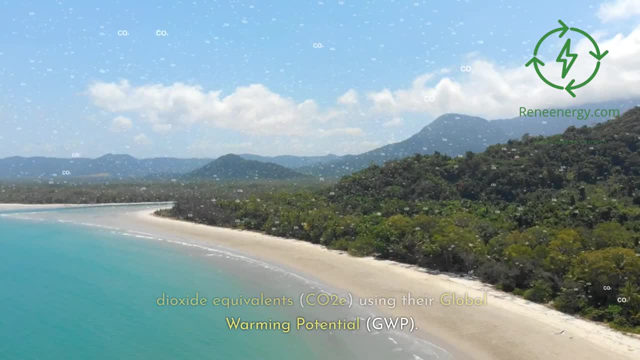 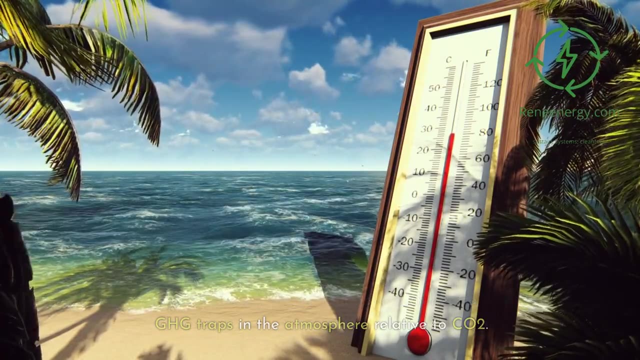 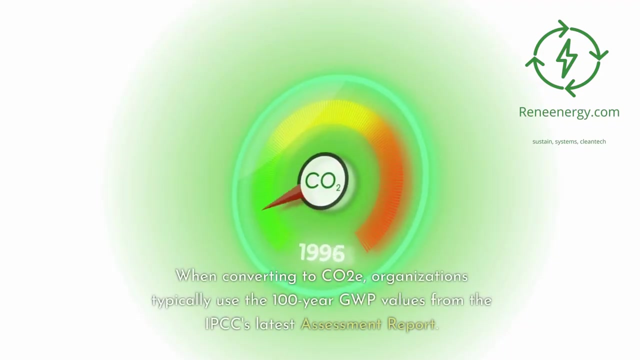 equivalents using their global warming potential. The GWP is a measure of how much heat a GHG traps in the atmosphere relative to CO2.. The IPCC provides GWP values for different GHGs. When converting to CO2e, organizations typically use the 100-year GWP values from the IPCC's latest assessment report. 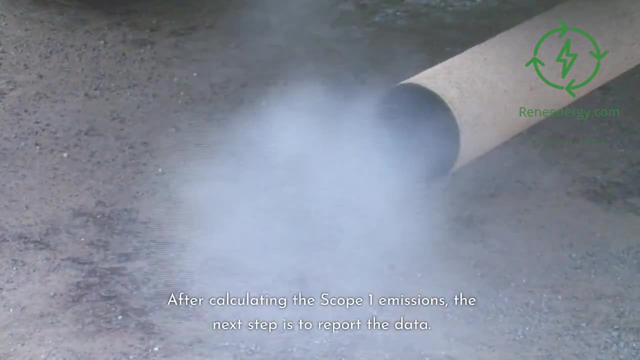 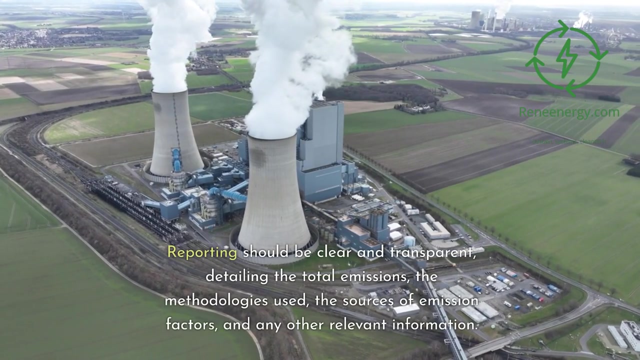 Step 6. Report & Verify. After calculating the scope 1 emissions, the next step is to report. the data Reporting should be clear and transparent, detailing the total emissions, the methodologies used, the sources of emission factors and any other relevant information. 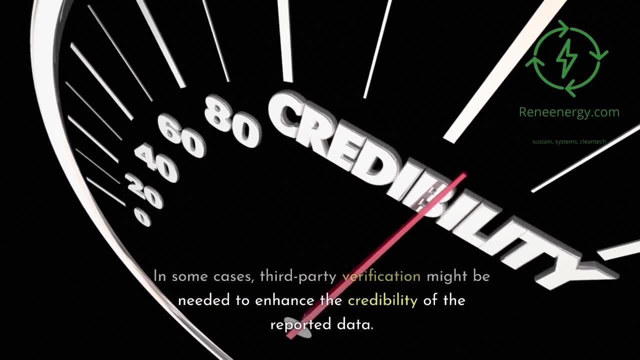 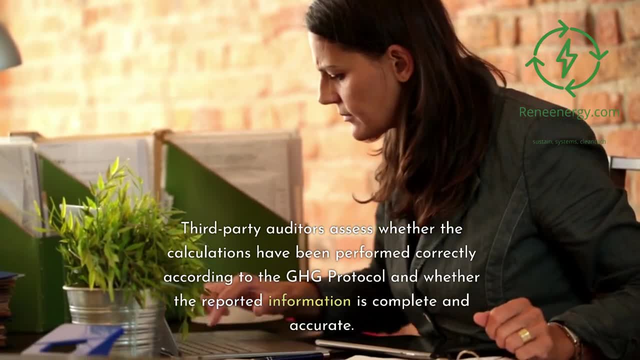 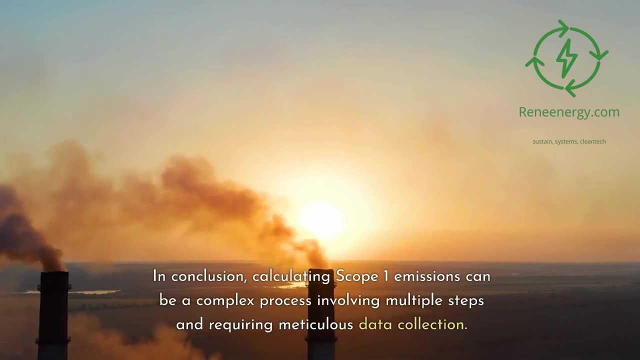 In some cases, third-party verification might be needed to enhance the credibility of the reported data. Third-party auditors assess whether the calculations have been performed correctly according to the GHG protocol and whether the reported information is complete and accurate. In conclusion, calculating scope 1 emissions can be a complex process involving